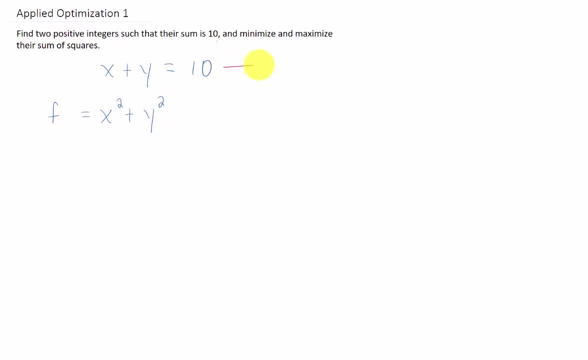 But since this is Calculus 1, we only want to deal with one variable. That means that we should solve this equation for, say, y, which would be 10 minus x, and then take that result and plug it into our sum of squares formula, which we're trying to maximize here. 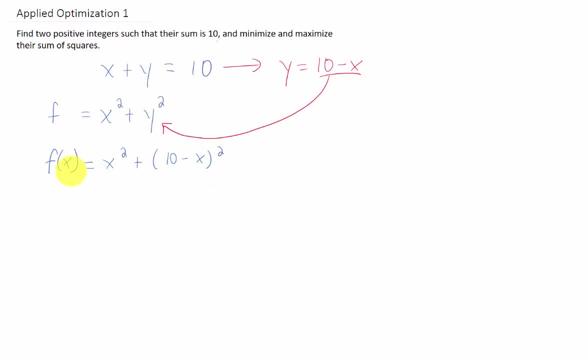 Now this function is a function of just x, It's a function of one variable, whereas before we had a function of x and y, And we can maximize and minimize a function of one variable. Now we should have an interval for this. This situation says that we have two positive integers, such that their sum is 10.. 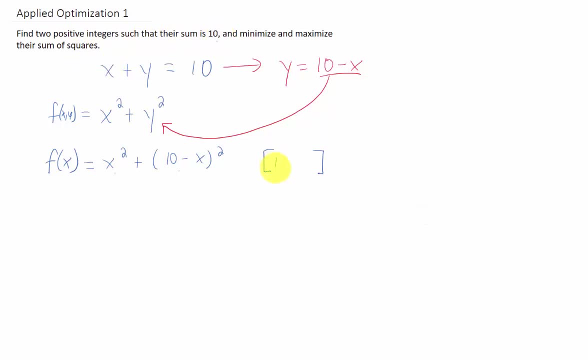 So the smallest possible value that we could have of x would be 1, and the largest possible value of x would be if x was 9 and y was 1.. Notice that x can't be 0, because it has to be positive. 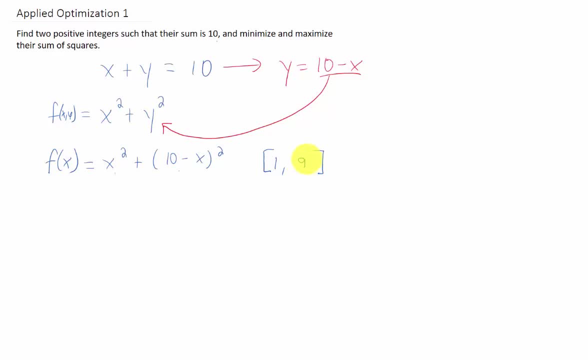 Notice that x cannot be 10, because that would make y 0, and y has to be positive. Okay, now let's optimize this function. That just means find an absolute max and min. So we should take a first derivative of this function. 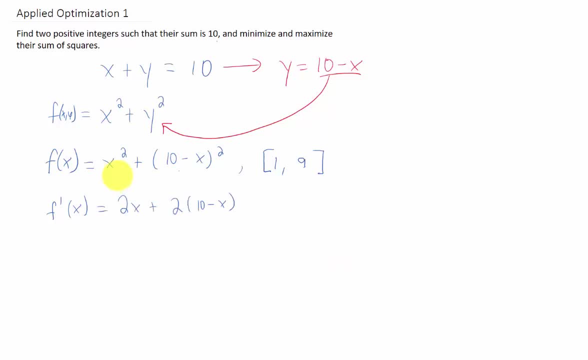 and set it equal to 0 to find our critical points. The derivative of x squared is 2x. The derivative of this second term involves a power rule. we bring the 2 down, we make the power on 10 minus x, 1,. 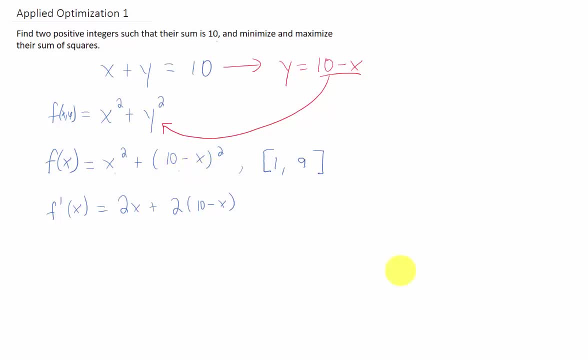 but then we have to multiply by the derivative of the inside function, which is negative 1.. So let's write this derivative out and see what we got. I'm going to just start by multiplying this negative 1 by this term, which makes this plus and minus. 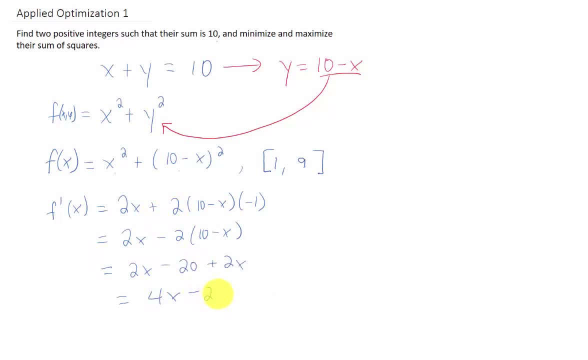 Now let's distribute and I'm getting 4x minus 20 as our first derivative. Now if we want critical points, we have to set that first derivative equal to 0.. If we add 20 to both sides and divide by 4, we get that x equals 5 is a critical point of this sum of squares function. 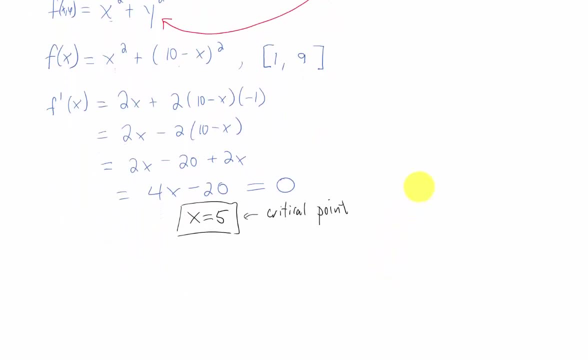 Now, to find the maximum and minimum values of this function, we just need to plug in the critical point and the two endpoints of our interval. That means: let's find f, f and f- f is going to be 1 squared plus 10 minus 1 squared. 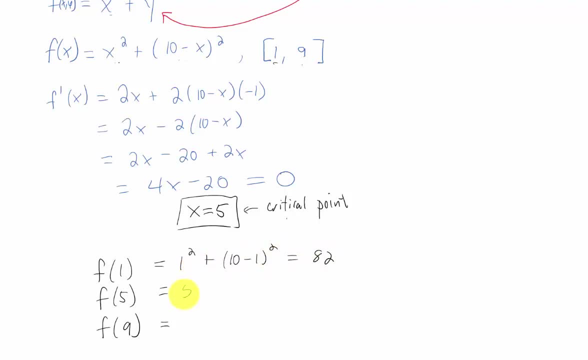 Which, if I'm not mistaken, is 82.. f is going to be 5 squared plus 10 minus 5 squared, which should be 50.. And f should be 82. So obviously, these two values of 82 are the maximum. 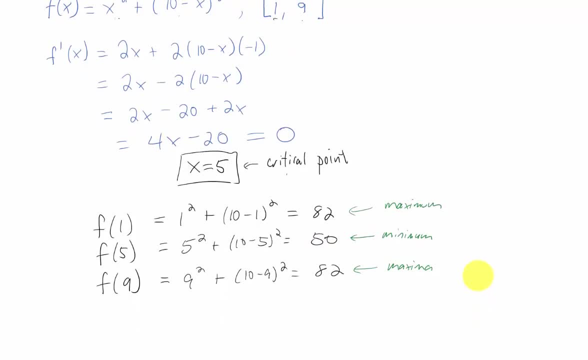 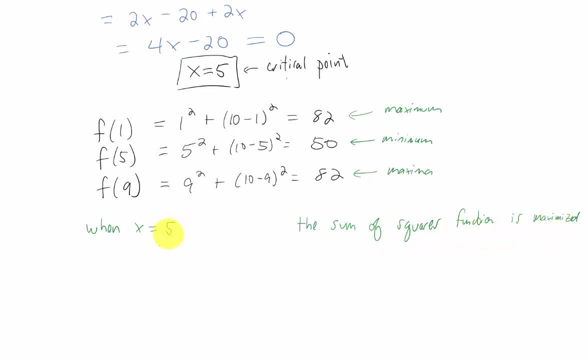 and this value of 50 of our function is the minimum. So let's take that and summarize the answer: When x equals 5, the sum of squares function is maximized, Because we know that the two integers have to add up to 10,. 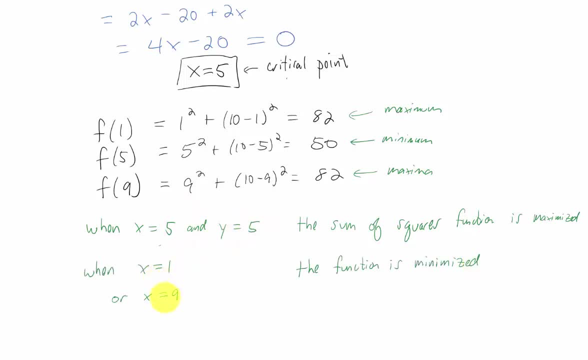 we can conclude that y is 5 as well. When x is either 1 or x equals 9,, the function is minimized, And when x is equal to 1,, y would have to be 9.. And when x is equal to 9,, y would have to equal 1.. 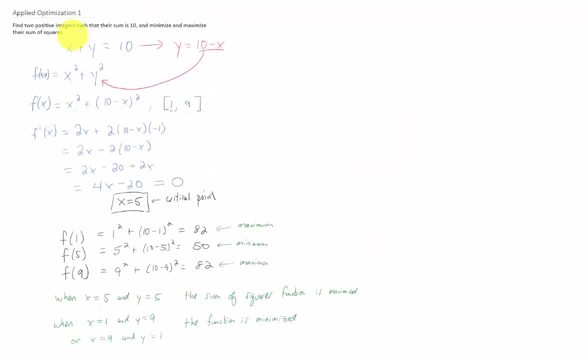 So let's go back to the original problem. We have two positive integers, such that their sum is 10.. We want to maximize and minimize their sum of squares. Well, we found that when the two integers are 1 and 9, the sum of squares 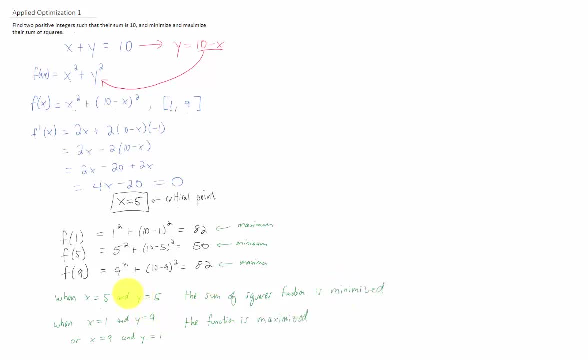 Oh, it looks like I wrote this backwards. Yep, so I wrote that backwards. When the two integers are 1 and 9, the sum of squares function is maximized, And when the two integers are 5 and 5, the sum of squares is minimized. 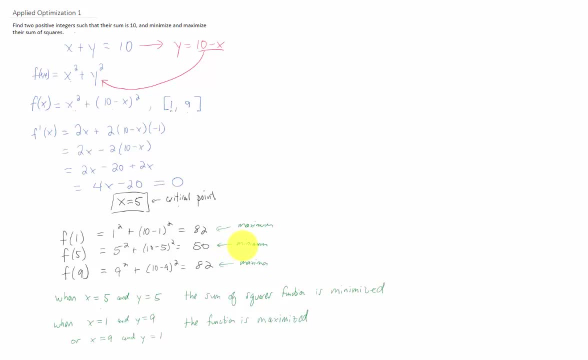 Okay, sorry about that slip up at the end, but this looks correct now. 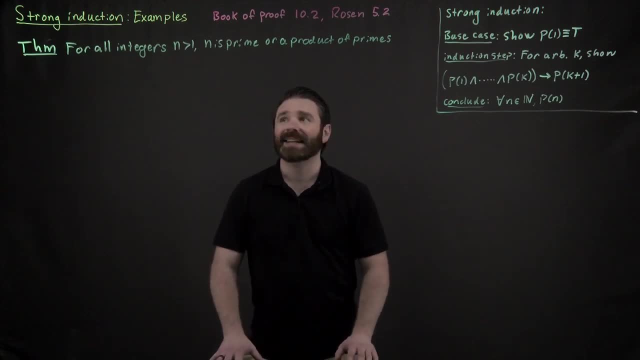 So let's look at our first example of strong induction in action. So here we have a theorem, and this theorem says: for all integers greater than 1, it's either prime or a product of primes. And if you haven't heard of primes or seen their definition, please see the side video. 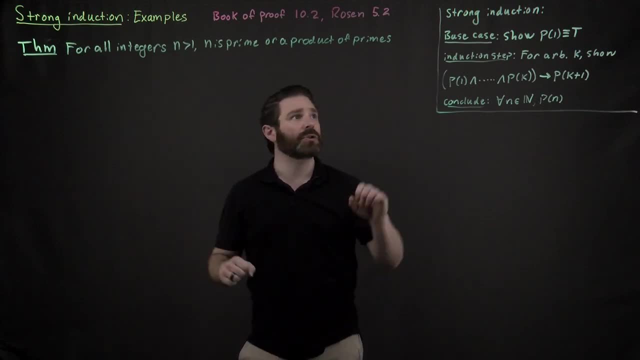 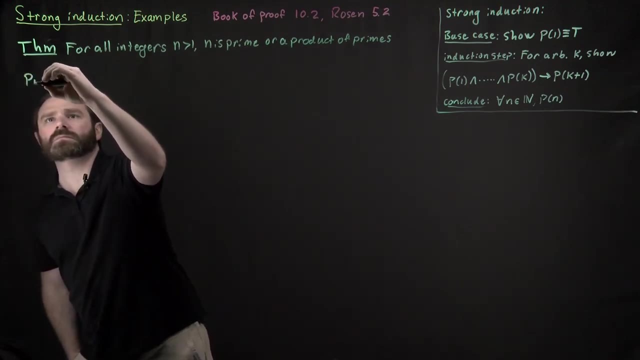 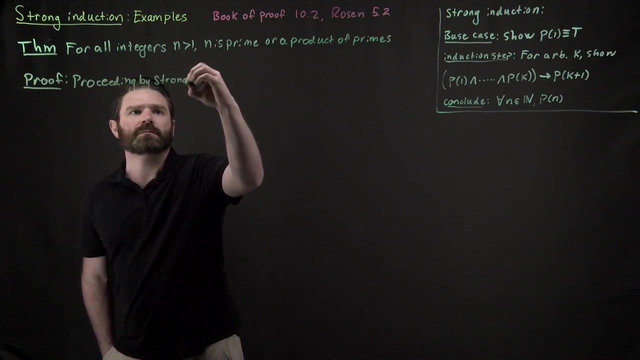 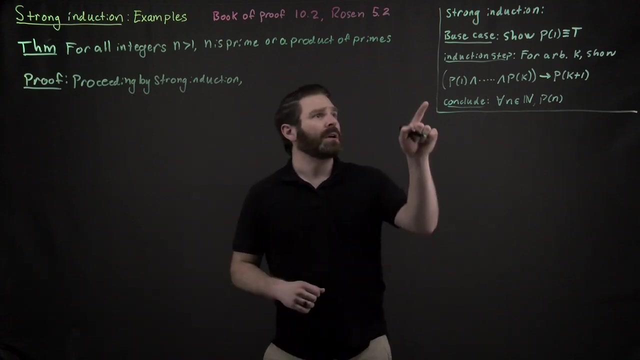 But in any case, we want to try to prove this statement here using strong induction. So let's go ahead and start out our proof So, proceeding by strong induction. we have to show a base case And, just like previously we saw with normal induction that there comes in two different flavors. 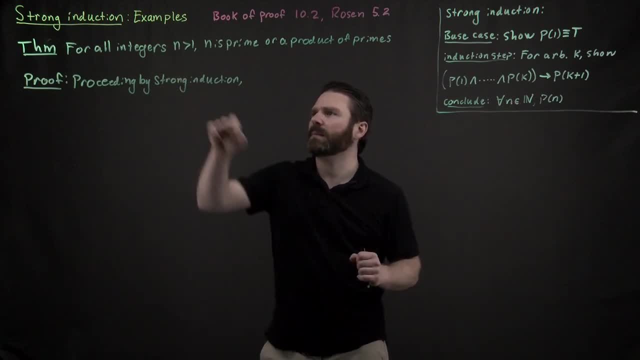 you don't just have to talk about all natural numbers Here. indeed, we're not talking about all natural numbers, We're talking about those that are greater than 1.. So, similarly, similarly to how, in that previous definition 2 of normal induction, we had the ability to prove statements for sets other than n-